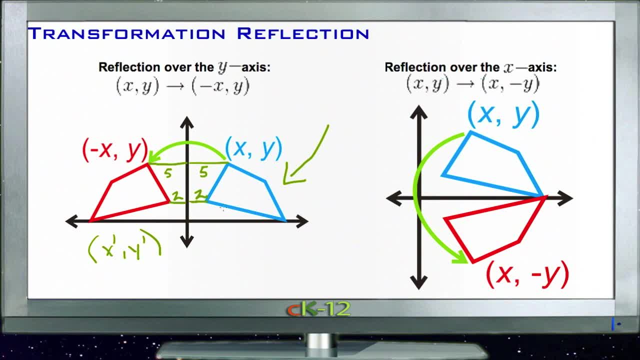 it's just going to be on the other side of the reflection. yeah, And we can do that, but sort of shorthand for that is by taking each location, each point, whatever the coordinates are- X, Y- and then translating them by making the X coordinate negative and not changing. 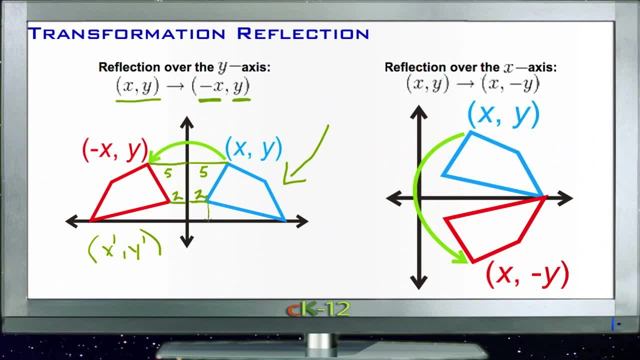 the Y coordinate. So for instance, if this point here was say 2, 2,, then the new point would be negative, 2, 2.. Negative 2, positive 2.. So we just change the X coordinate without. 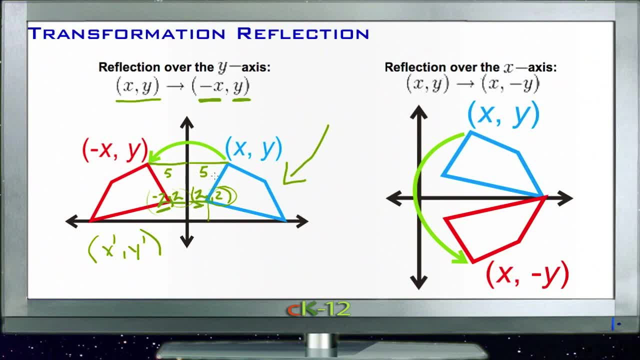 changing the Y coordinate, It stays the same. Yeah, This one would go from say maybe this is 5, 9, then this one over here would be negative 5, 9.. The Y coordinate stays the same, whereas the X coordinate becomes negative. 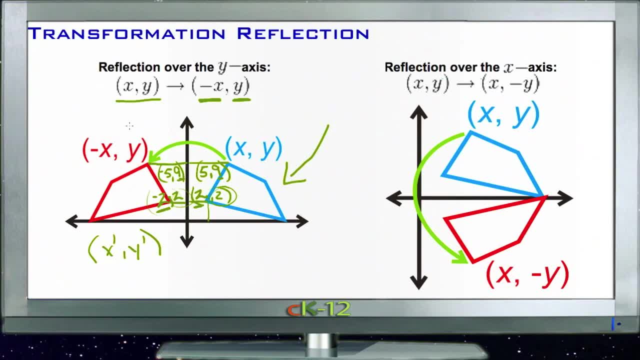 So that's all we have to do to reflect over the Y axis, just change the sign of the X coordinate To reflect over the X axis, which seems, I know, a little backward, because we think the X axis runs left to right. Y is a vertical flip related to the X axis. 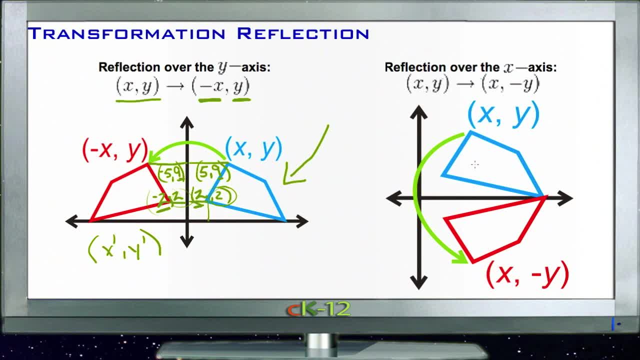 But that's because we're talking about putting the mirror in horizontally, so that the image then changes vertically. So then, to do that one, we just do the opposite of what we did to reflect over the Y axis, whereas the Y axis, we change the X coordinate To reflect. 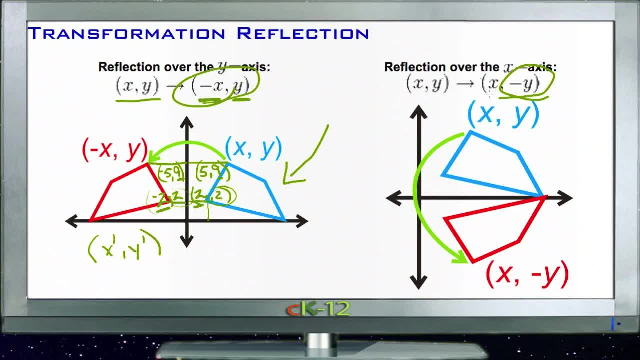 over the X axis, we change the Y coordinate. So now the X coordinate stays the same, the Y coordinate becomes negative. So, whatever these things are, say this point over here. we'll say this one is- I don't know- 9, 5.. 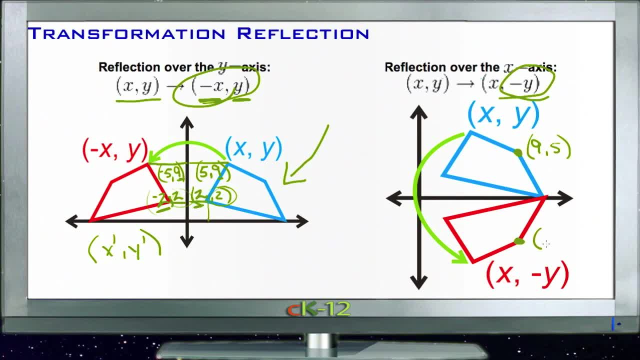 To reflect it, that corresponding coordinate down here would be 9, negative 5.. So now the X coordinate stays the same and the Y coordinate is the one whose sign changes. So to reflect over the X axis, keep the X coordinate the same. To reflect over the Y axis, keep the 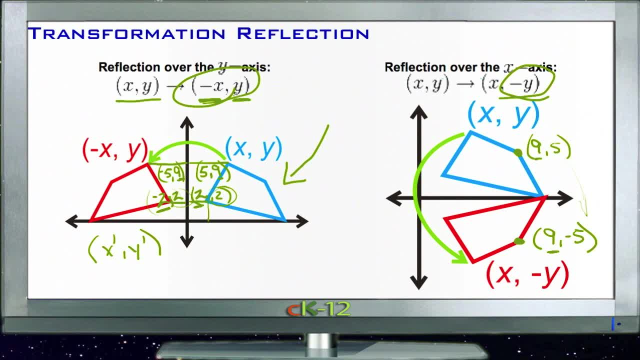 Y coordinate the same. That's how I end up remembering it myself. I just remember that I'm not changing the coordinate that goes with the axis I'm reflecting over. Cool, All right, let's take a look at the example. All right, let's take a look at the example.